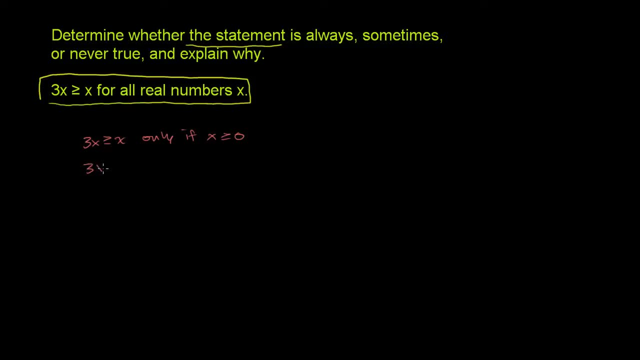 It is not true for all real numbers. 3x is greater than or equal to x is not true. Not true for all real numbers. And the reason why I say that this was kind of a strangely constructed question is: I think the goal of the problem, writer, is that they wanted us to write sometimes, which is what we did in the last videos. 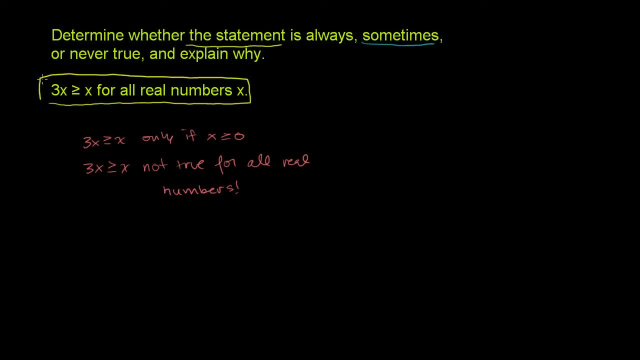 But if you say sometimes you're actually interpreting this as the statement, Not the whole thing. You could say that 3x is greater than or equal to x, sometimes for certain real numbers. Sometimes This is true. You can say this is true sometimes. 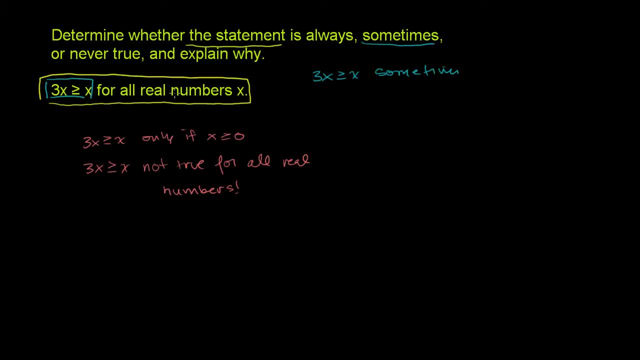 But this whole thing- 3x is greater than or equal to x for all real numbers- is not sometimes true and sometimes not true. This is never true. You can never say it's for all real numbers. It's not like this is true on Monday and then on Tuesday this becomes not true, and then on Wednesday it becomes true. 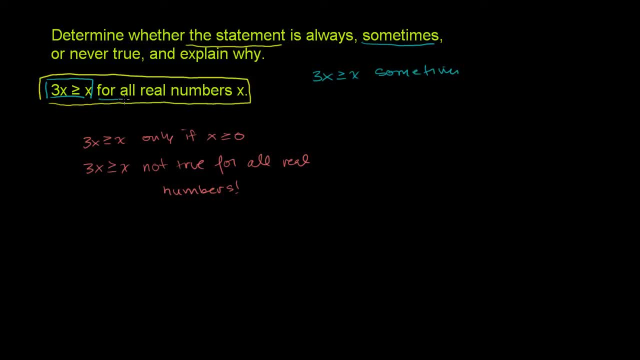 This is never true. This statement for all real numbers just won't work. You can't say for all real numbers: 3x is greater than or equal to x. I hope I'm not muddying up the issue here, But I want to make it very clear, because this statement is a false statement. 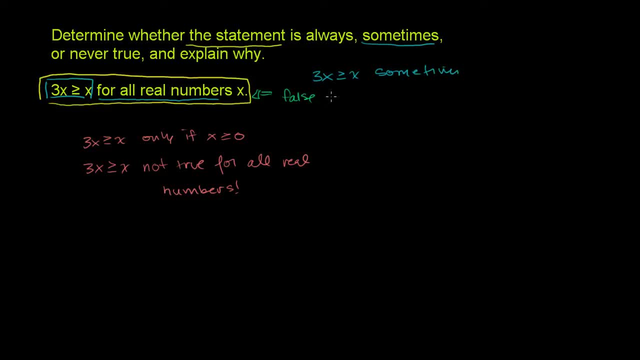 This is a false statement. So, if you really want to think about it, if you view this whole thing as a statement, this statement is never true. It's not like it's true on Monday and then all of a sudden not true the next month after that, or all of a sudden it becomes true again. 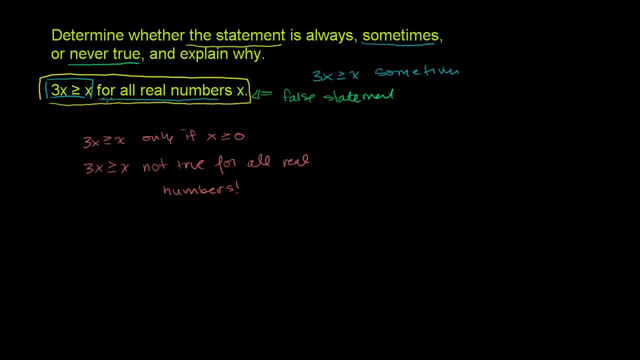 No, It's never going to be true. I don't care how long you wait or how far in the past you go, This statement will never be true. that 3x is greater than or equal to x for all real numbers, x. The problem writer wanted us to circle sometimes because, as I already stated, and I'm maybe getting a little repetitive here- 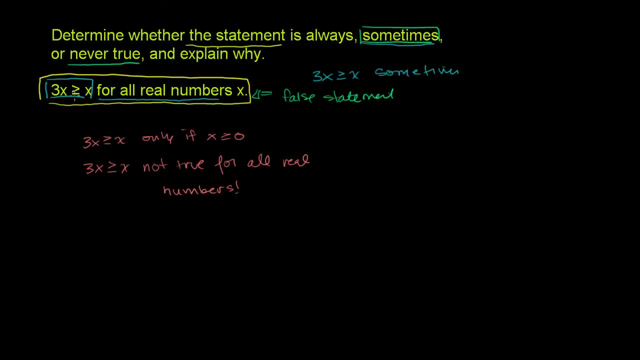 because I think they wanted us to think about the statement as 3x is greater than or equal to x. So my general opinion: I mean 3x is greater than or equal to x, sometimes for some real numbers, but not for all real numbers.